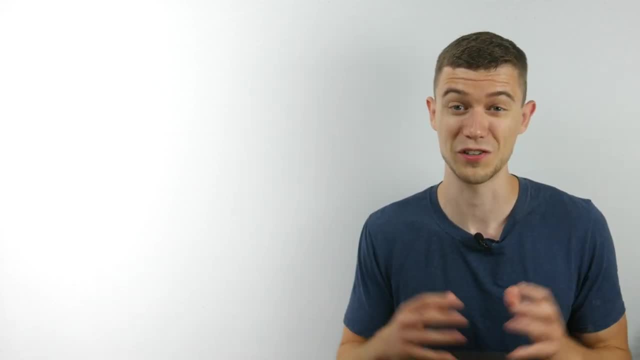 that's when I started my math tutoring career journey. whatever you want to call it, Being able to go through college being a peer math tutor is such a great resume builder, regardless of what job you want to do after school. In my opinion, it looks like a much. 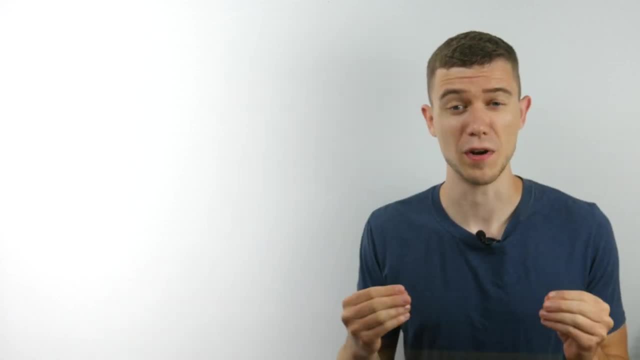 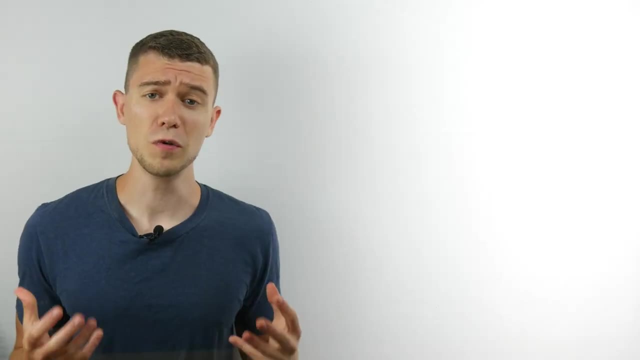 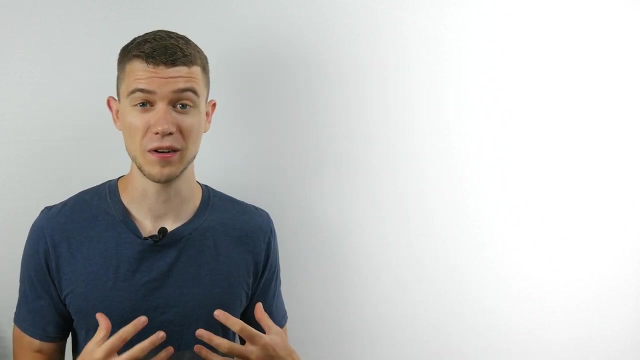 more professional position. It's just a nice thing to have on your resume that sort of diversifies you and sets you apart from your competition for whatever job you're applying for. Third, I wish I knew how flexible the schedule was that I could have and work with- At least in my experience- every single tutoring position. 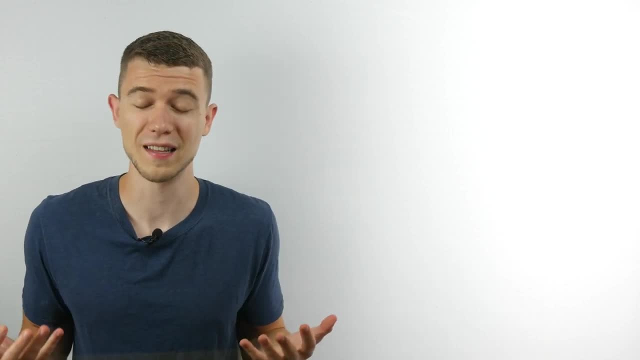 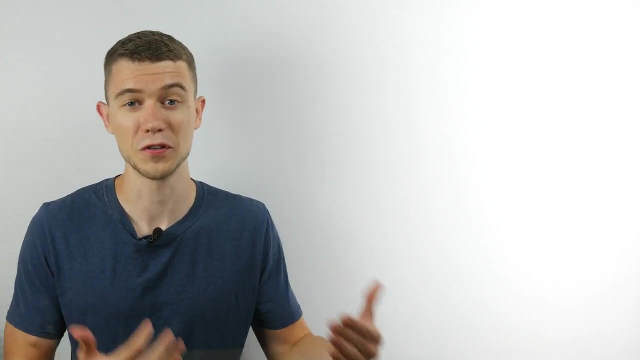 I've had- and I've held a few- have more or less allowed me to pick my own schedule. Now, obviously, you can't work wild hours and you need to be able to work when students are available so they can come and see you, But as long as you're getting your hours in every week. 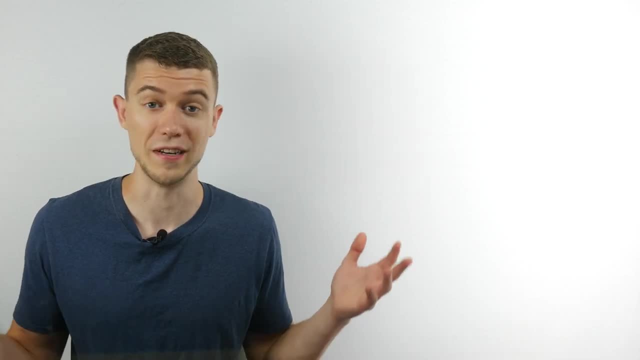 I was able to just sort of set my own weekly schedule for each semester, depending on whatever else I had going on, whether that was class or maybe other jobs. I was able to just sort of set my own weekly schedule for each semester depending on whatever else I had going on, whether that was class or maybe other jobs. 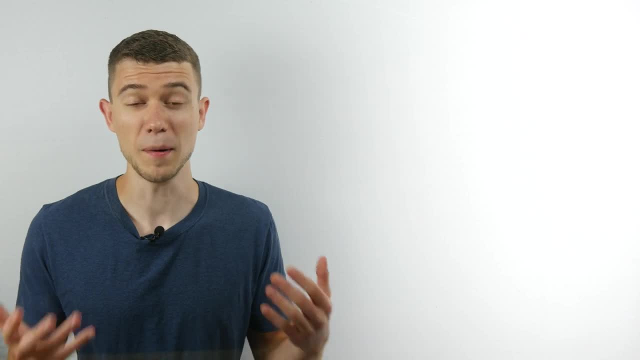 I was able to just sort of set my own weekly schedule for each semester, depending on whatever else I had going on, whether that was class or maybe other jobs. It's a very flexible position, especially if you get into online tutoring. Now we're talking about 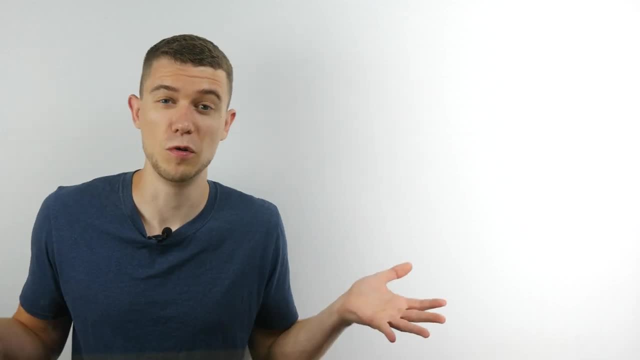 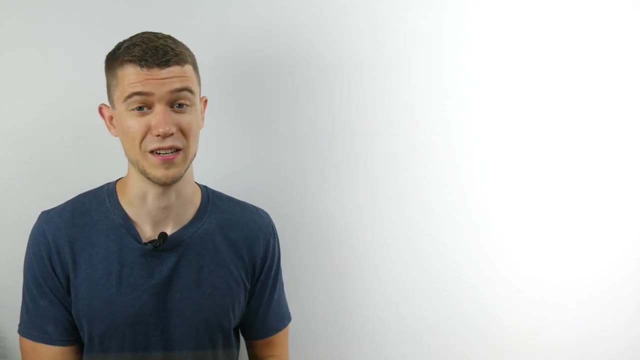 a lot of flexibility because you can wake up at whatever time you want and just get on your computer and start tutoring. So the flexibility with being a tutor is a really, really nice perk. The fourth thing I wish I knew before becoming a math tutor, specifically: 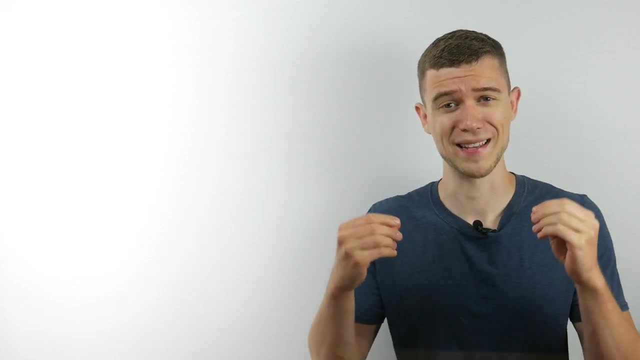 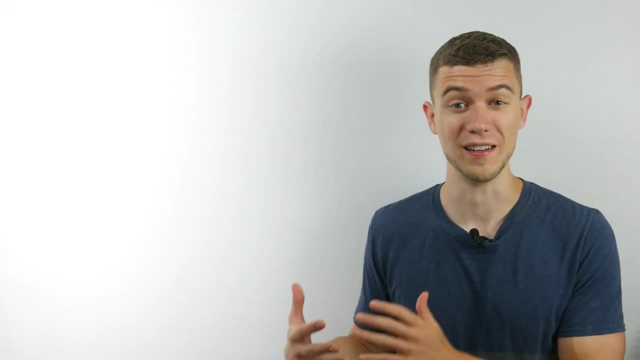 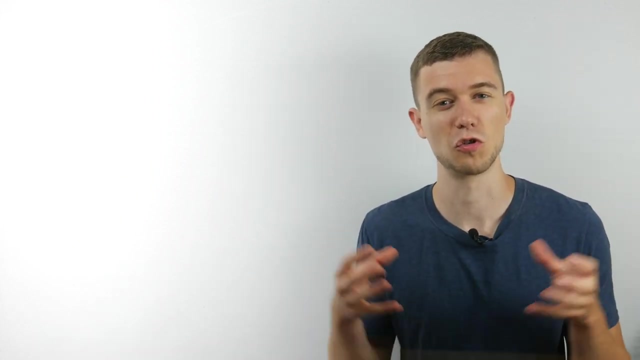 is. I wish I knew how much math I was going to forget when I started tutoring. It's funny when you start tutoring the subjects you did really well in in school and you realize how quickly that information fades. It took me a lot of time to be able to scrape up all the pieces of 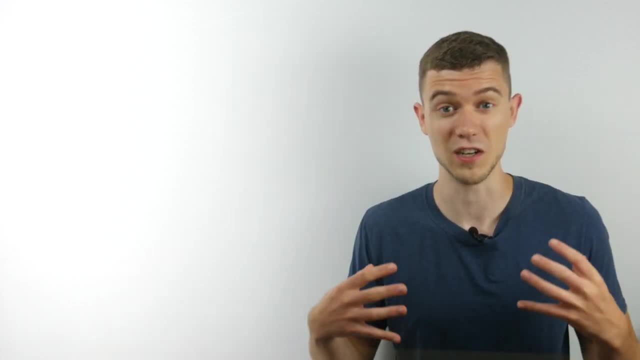 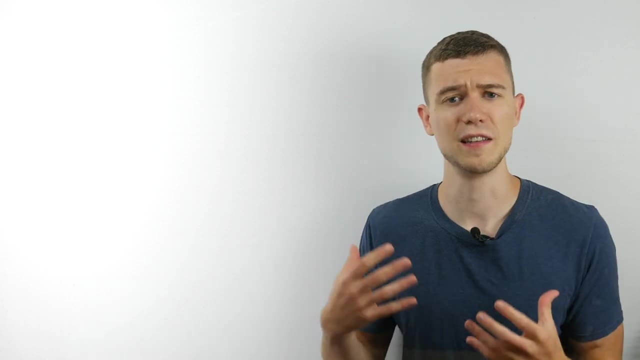 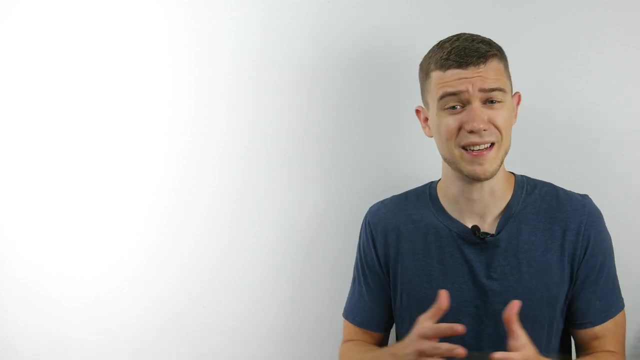 all the math classes I've had in the past and be able to just internalize that and help other people learn it as well. It's a really good idea to consistently be reviewing material that you're tutoring or anything. that's been a very long time for you, I know. for me it took a while. 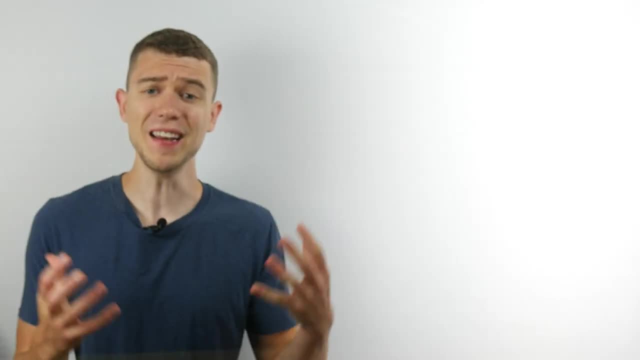 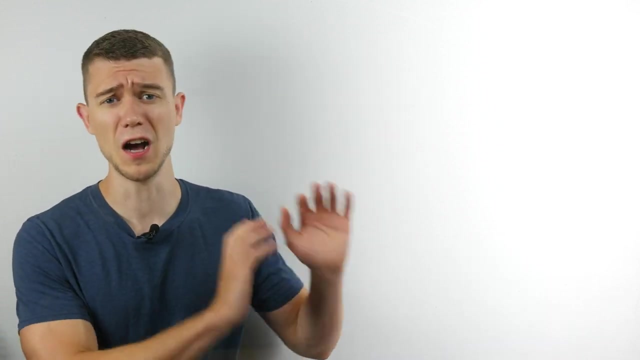 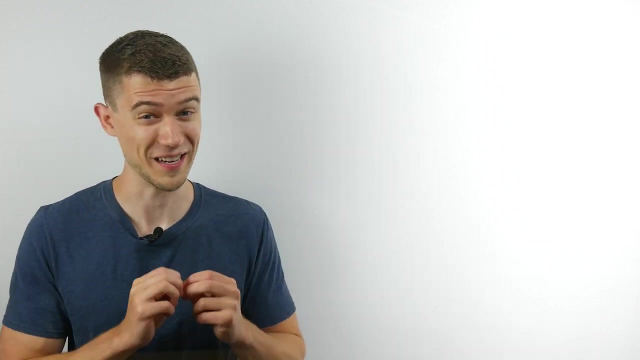 before I really was able to absorb everything Getting into working with students. the fifth thing I wish I knew before becoming a tutor was some students- not all students- are going to have a very high level of expectation for what you're going to do for them. as a tutor, I've had students 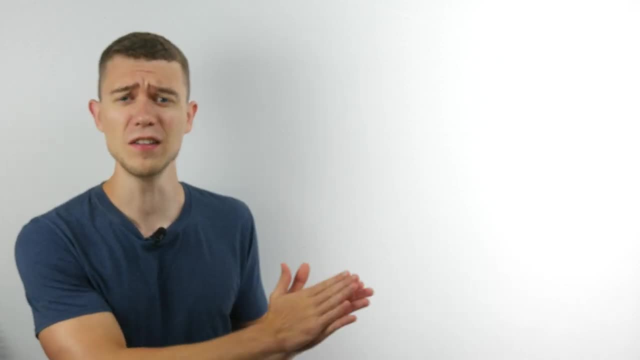 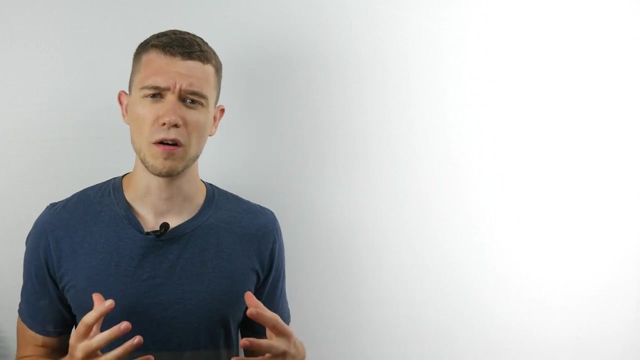 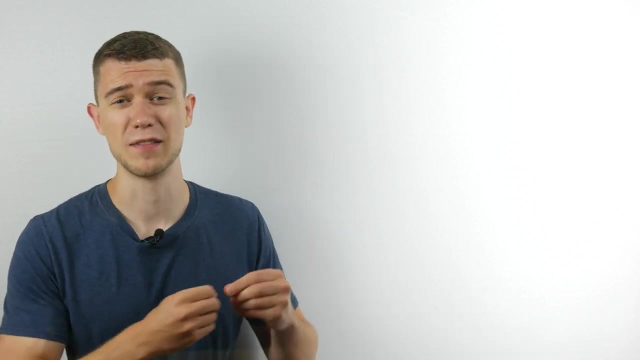 who want little to no help. and then I've had students who essentially want me to do all of their homework for them, while they sort of watch me do it. It's just something to be aware of that. some students will try to use every last drop of resource and energy that you have to. 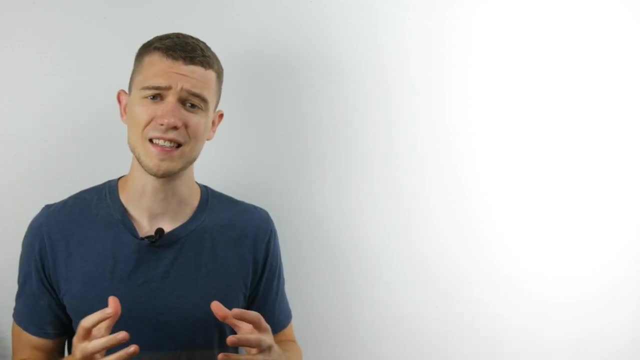 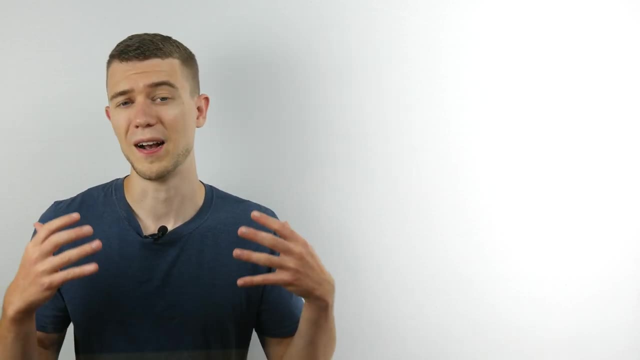 make sure they get their own work done. It's nothing against the students Now. this doesn't always happen, and after you have a few of these situations you sort of know how to deal with it. but I just wish I knew how many students really wanted a lot of hand-holding and they wanted a. 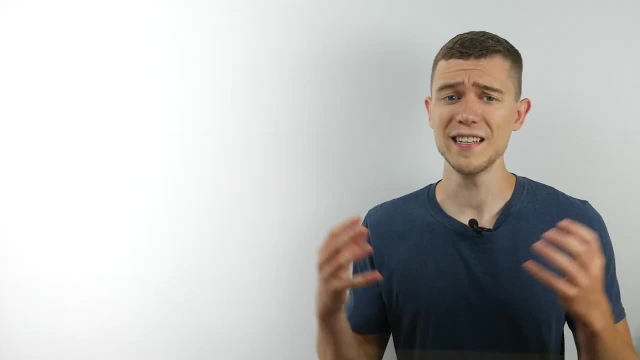 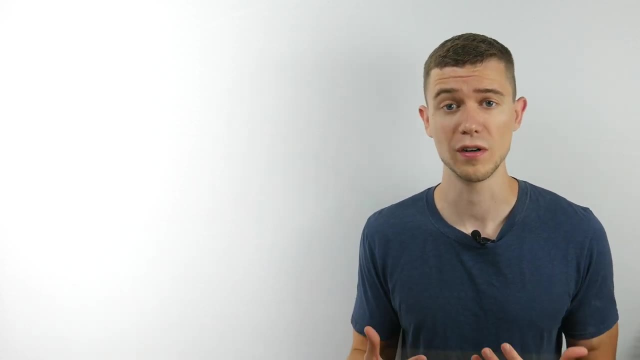 lot more help than a regular tutoring session should be. The sixth thing I wish I knew before becoming a math tutor was how many students are going to be able to do a lot of hand-holding. Some students are very, very reluctant to see tutoring. In fact, they almost see it as a sign. 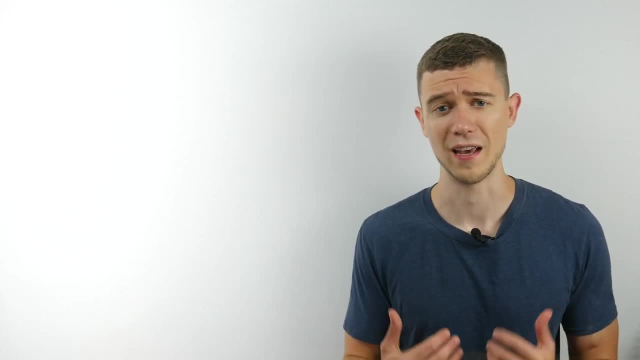 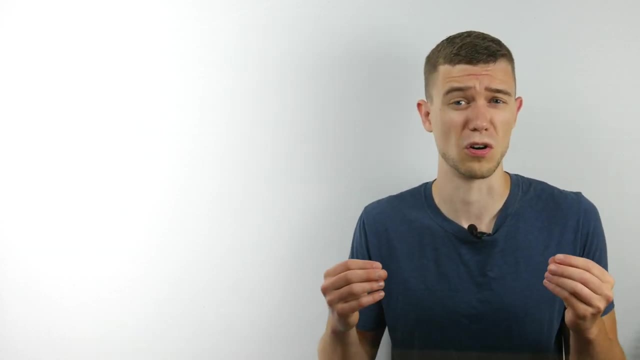 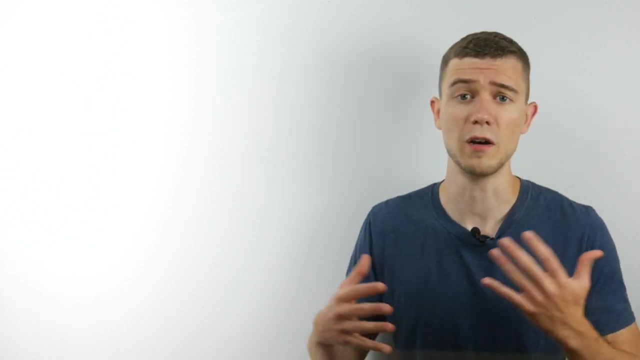 of weakness. I know I sort of felt this myself before I became a tutor. I sort of thought going to tutoring was something that students were only really struggling are supposed to do. but I found that even when I was doing well in a course, going to tutoring just helped me that much more Helped. 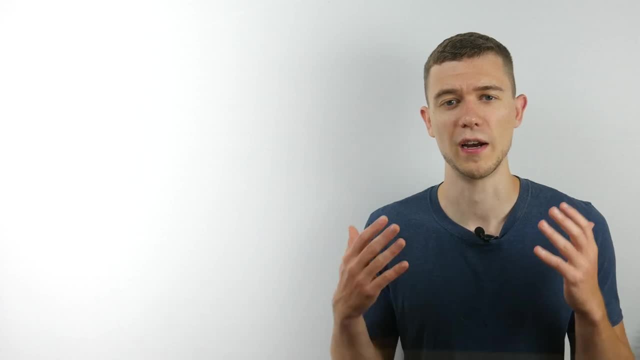 me solidify things and I think I wish I knew how many students really wanted a lot of hand-holding, How many students would be so reluctant, even when they were a good student and it could benefit them so much. So I like to tell students that tutoring really is for everyone. In fact, I think 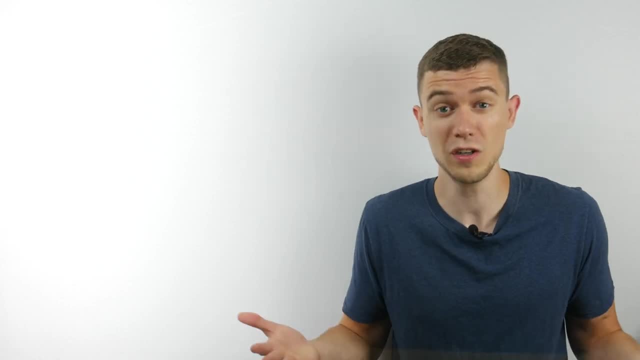 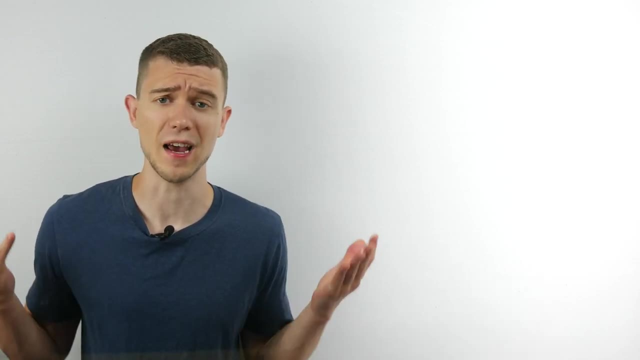 the best students out there go to tutoring and should get tutoring. Seventh thing I wish I knew before becoming a math tutor was how different every student is. Every person is different and the way they learn is different For different students. you're going to have to take a totally 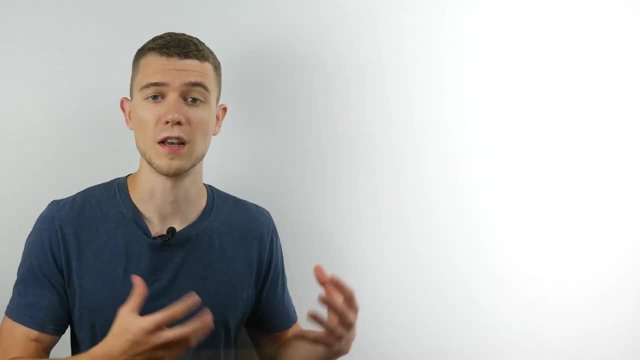 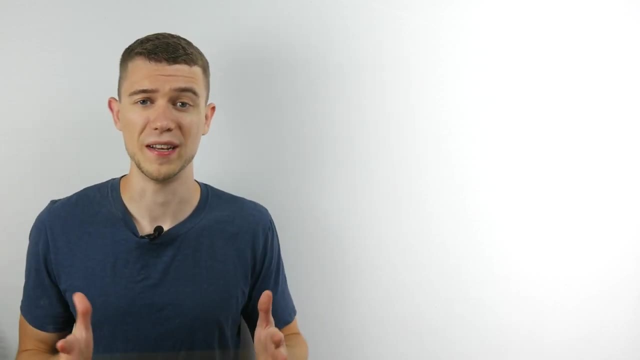 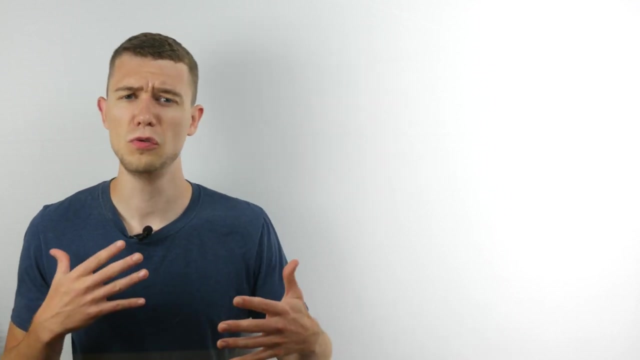 different perspective on how you teach them. Some students are much more visual, Some students are not. Some students are quick learners and some are not so quick. There's many different ways that students absorb information and the rate at which they absorb it, And so, as a tutor, you 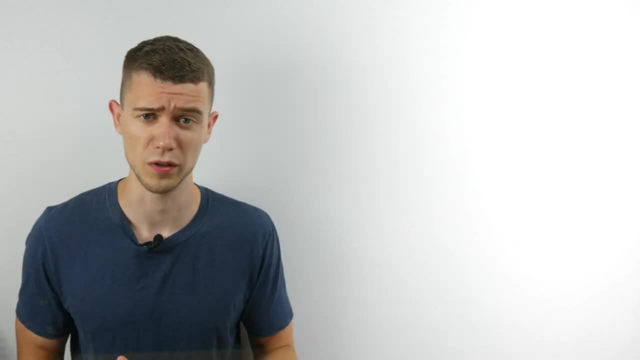 can sort of get an intuition for this. as you start talking with a student and working with a student, You know you kind of can gauge how fast you should go with things, How much information you should say That sort of thing. But I didn't realize before I became a tutor just how tough it would be to work. 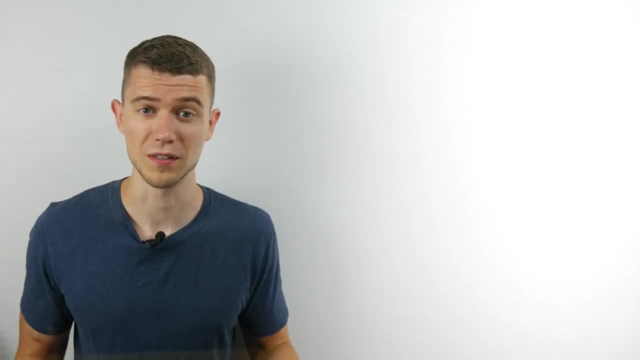 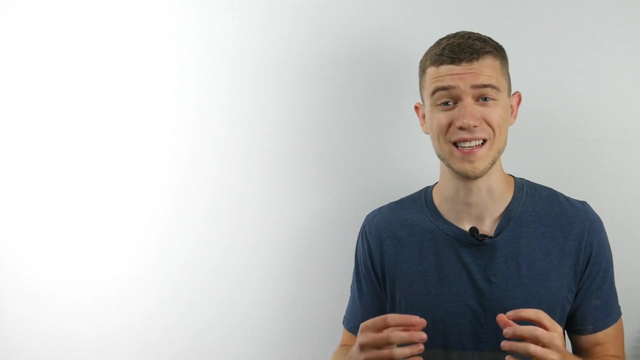 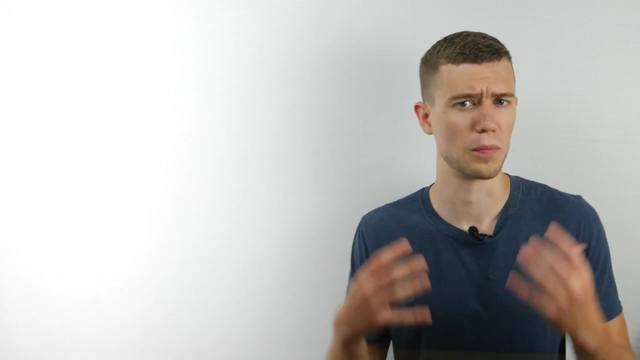 with so many different people on so many different levels. The eighth thing I wish I knew before becoming a tutor was how little training there was, At least in my situation. If you're planning on becoming a tutor, there might be a very standardized training program or process for. 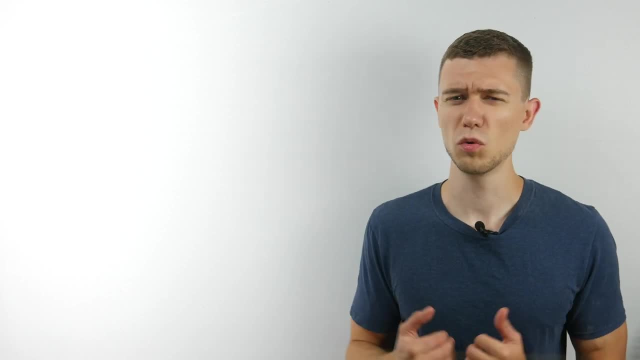 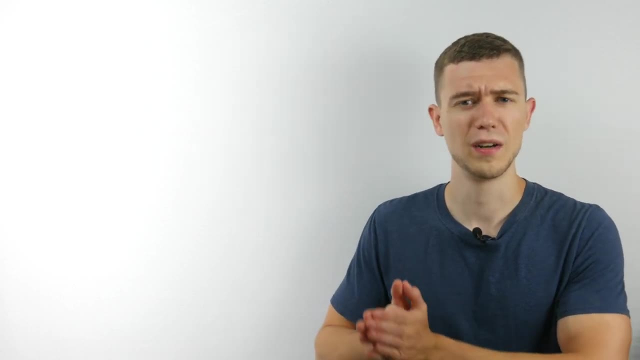 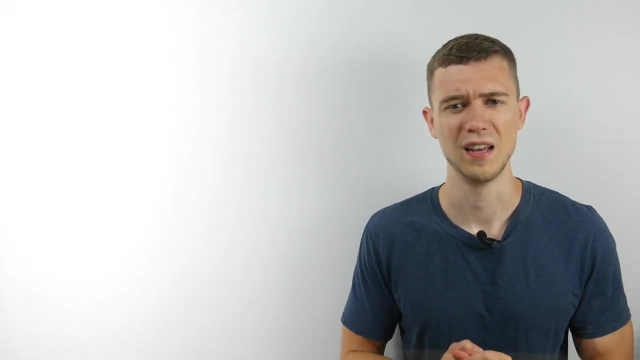 wherever you're looking at, But for me we did sort of have a training class kind of thing, But it wasn't so much about tutoring and tutorials. Much more of it was on learning habits and personalities and that sort of thing. It was just kind of like. 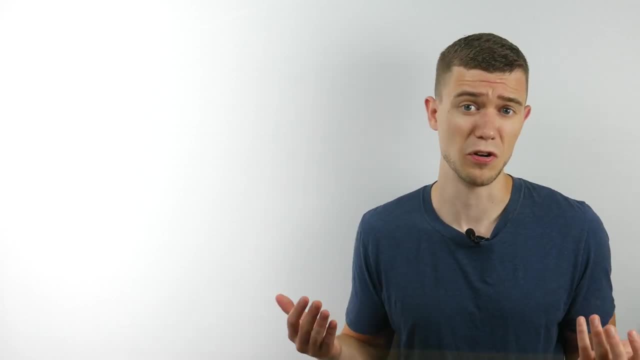 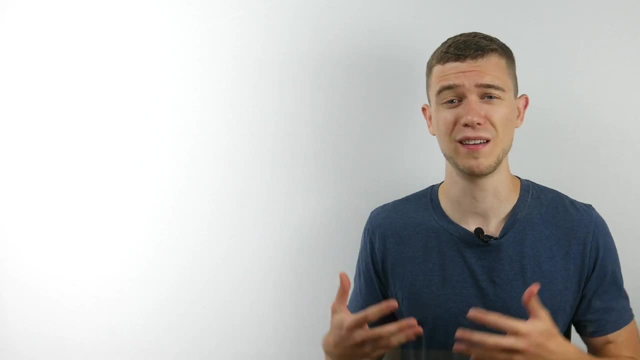 hey, you're a tutor. now Here's a student. You know the material right? Well, go tutor them, Not to say that there's a whole lot of training that can be done with tutoring. Everyone has their own field, their own technique and style, and so forth. 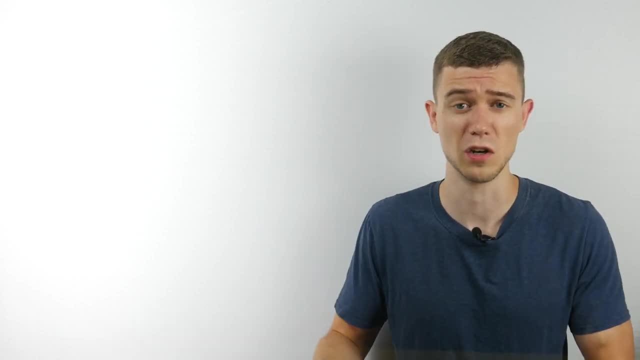 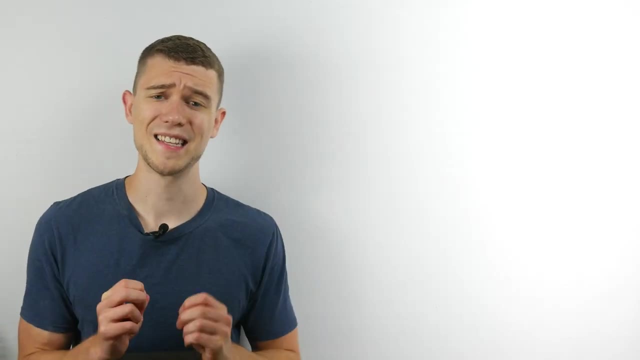 So it's not necessarily something you can train very much of, But I wish I knew that I was essentially going in blind and kind of having to find my own way. The ninth thing I wish I knew before becoming a math tutor is that students don't always know what they need help with. 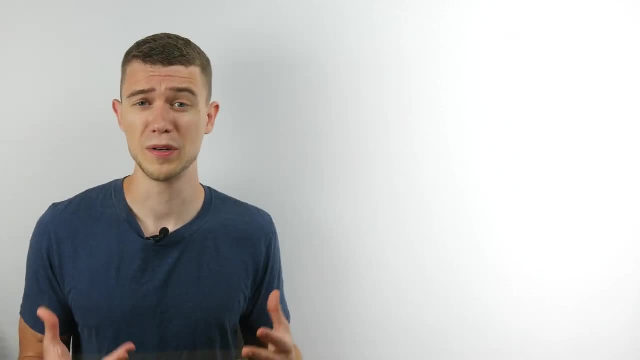 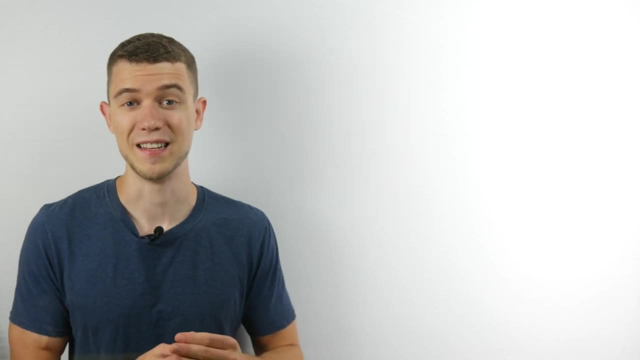 Students come to tutoring and maybe they don't know what they need help with. They just know they need help. I can't tell you how many times it's happened. A student comes to meet with me for the first time and they say: hi, I'm in college, I'm going to teach you math, I'm going to teach you. 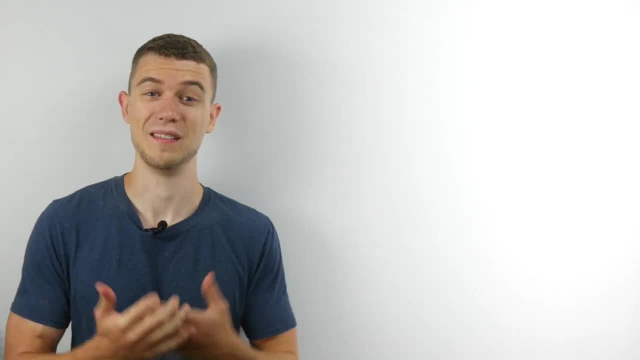 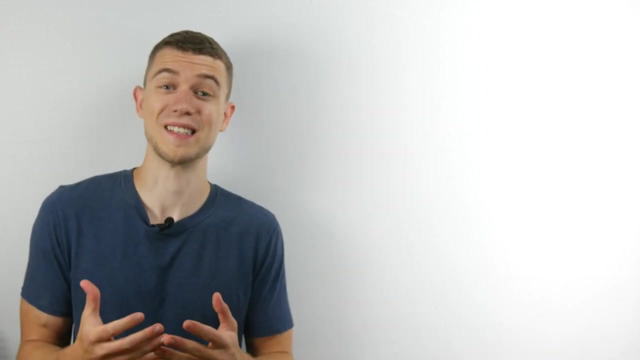 algebra and I need help. And I say, okay, great, What can I help you with? What things are you working on that you're struggling with? And they say, well, I don't know. Sort of just everything. And so that can be a little bit challenging to deal with Usually. if you look at some previous 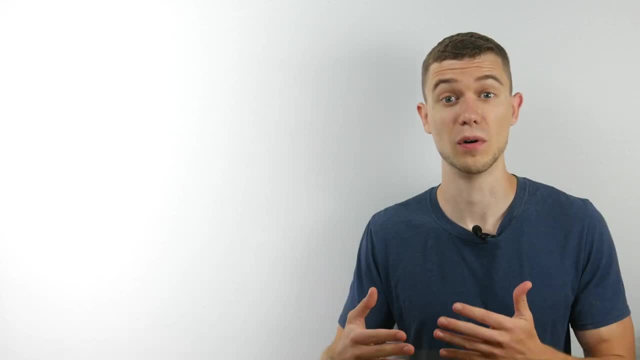 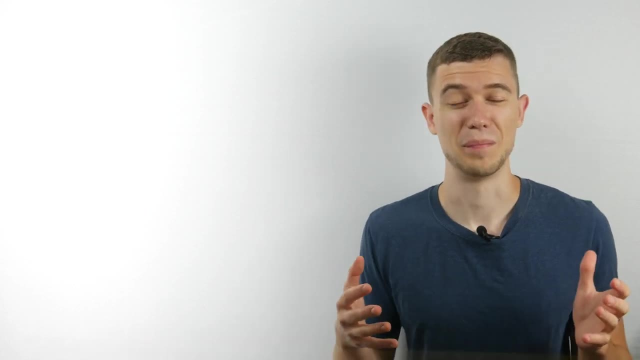 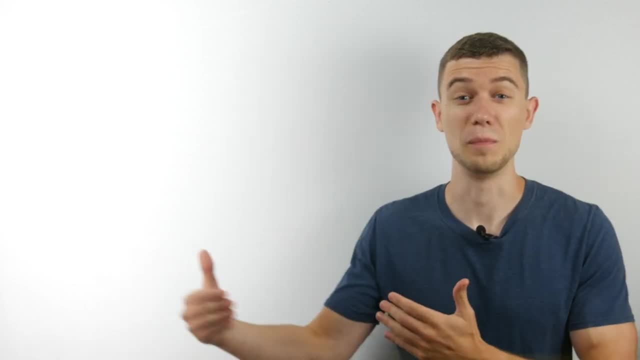 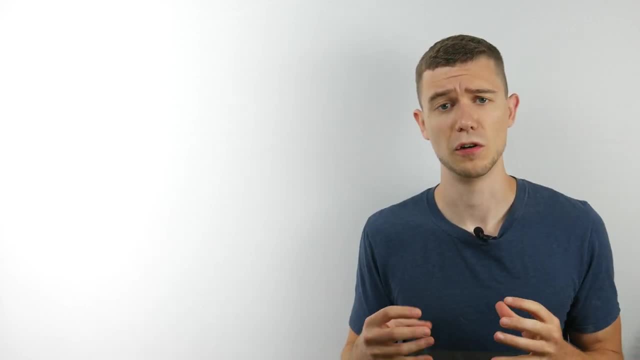 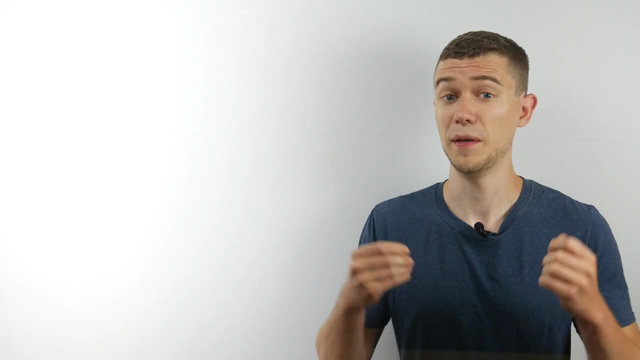 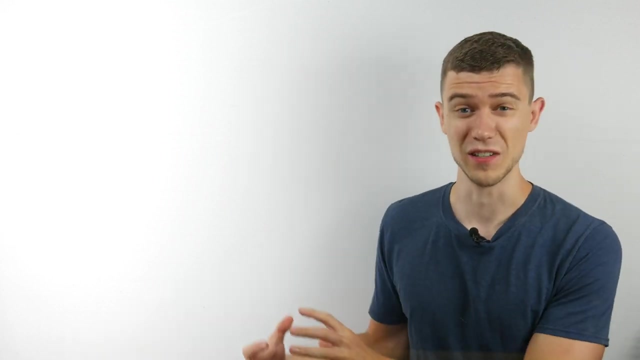 The eleventh thing I wish I knew before becoming a math tutor is that if you're tutoring for a college or university, the professors whose courses you are tutoring can be very picky. You know they don't want you doing problems necessarily a different way than their teaching. 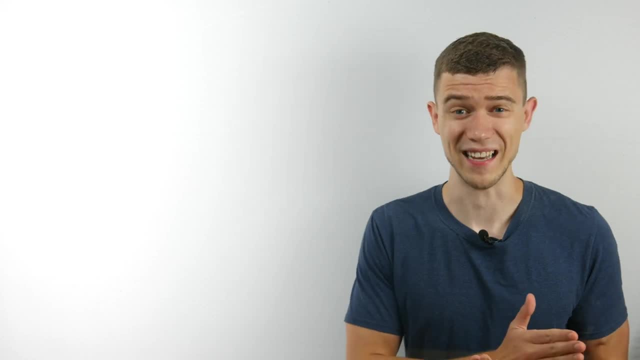 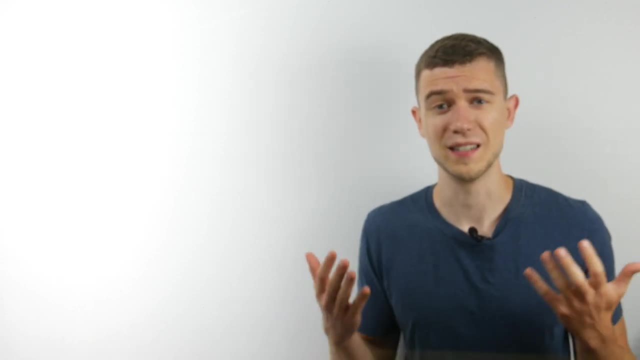 or they don't always want you using their past exams because maybe they reuse some of their content. some teachers don't even like you tutoring their classes at all, because they just want the students to learn from them, and that's it. this isn't something that happens all the time, but 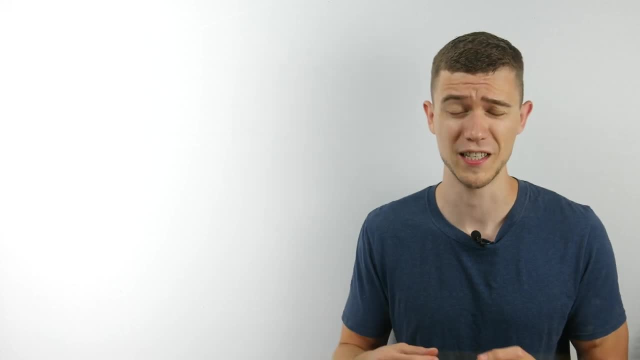 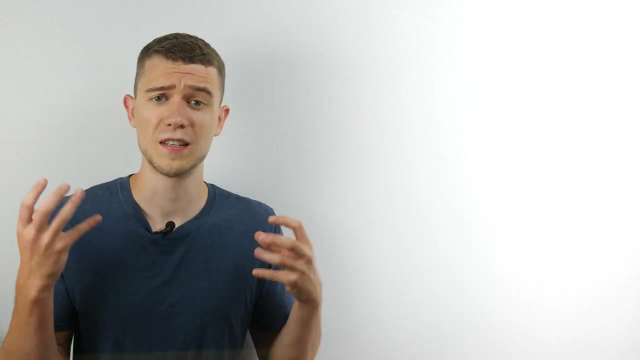 it's something to keep in mind if you're working at a college or university, that some teachers might want you to do things a very certain way or they might not want you tutoring their courses at all, depending on what it is next. i wish i knew that when you're a tutor, students sort of just. 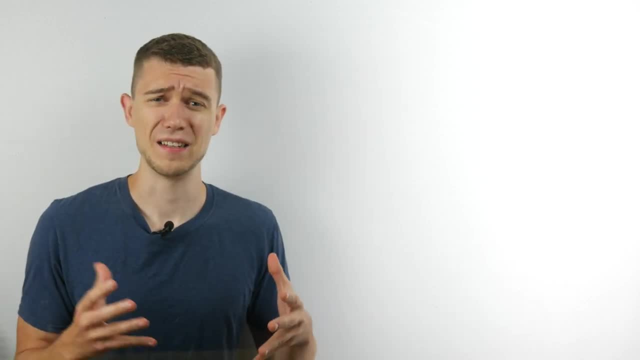 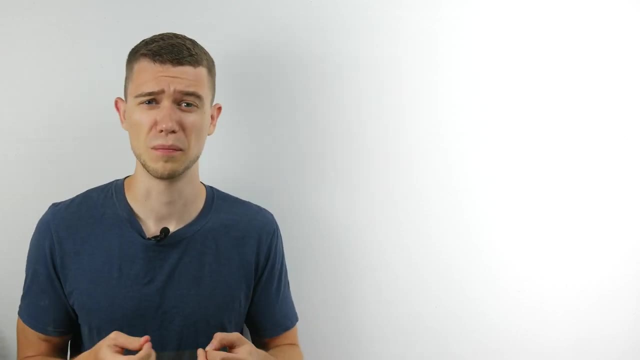 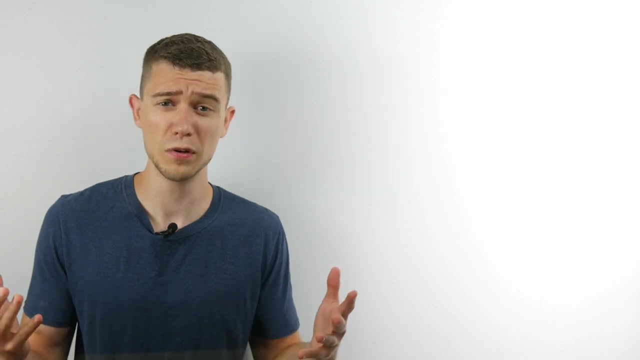 see you as this generic help thing, and problems can kind of come from anywhere. i've had students come to me with chemistry problems, physics problems, engineering problems, geology, class problems. i don't know anything about those subjects, but the fact that there's any sort of numbers involved or any sort of math involved. students can come and and i guess i can try to. 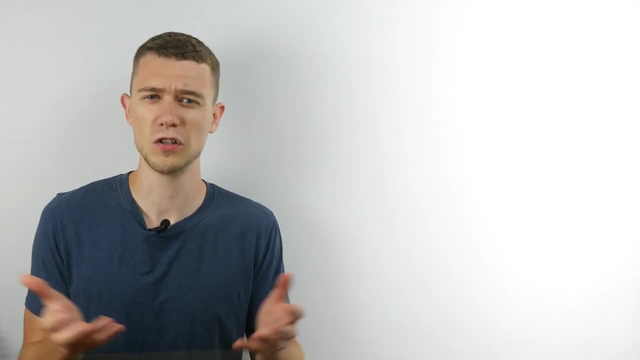 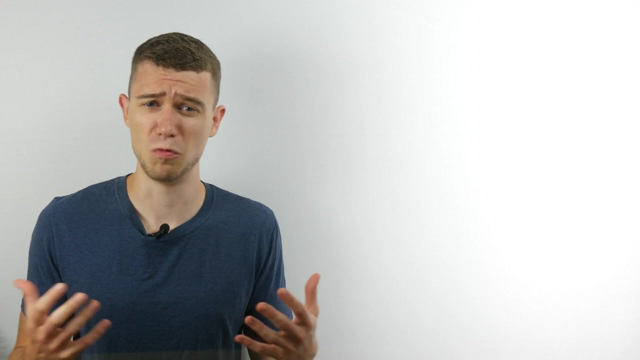 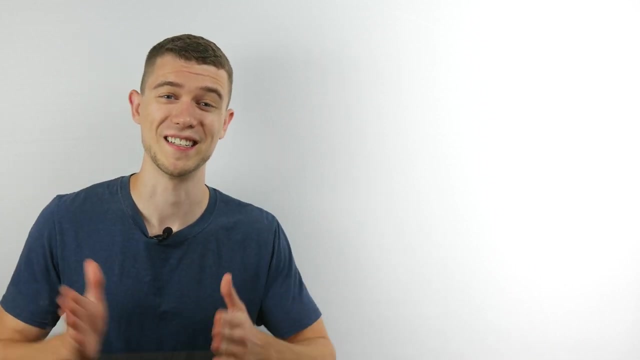 help them. i can't always. sometimes i can, but i never imagined just the vast number of problems students would bring to me, uh, for help. that i probably wouldn't have any idea. it's just something to keep in mind that when you're a tutor, students see you as a resource for more than just exactly what you're hired to do. 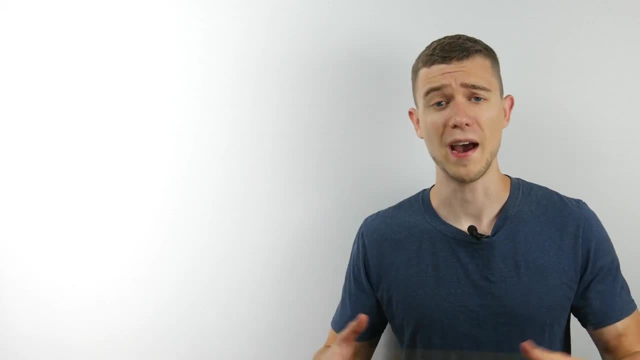 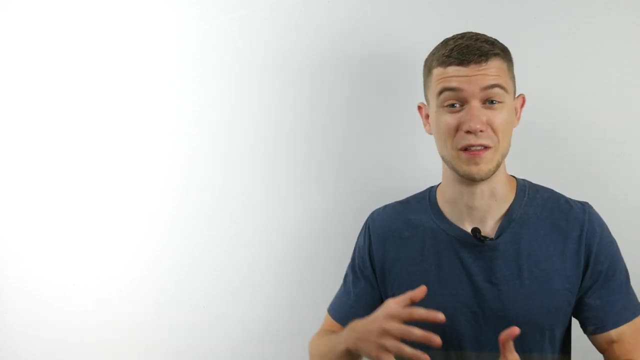 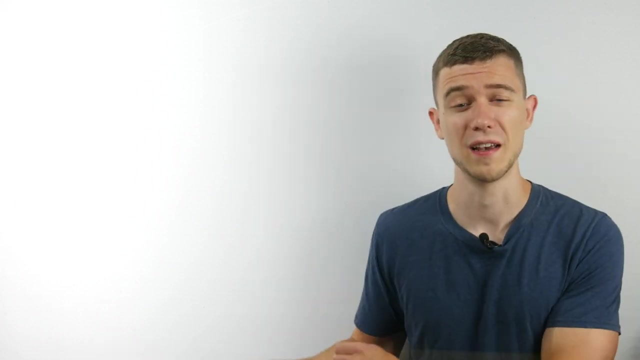 and also what i wish i knew becoming a math tutor was how rewarding it was going to be and also very fun. it's a very fun job. it's a very different job than many other things out there. you get to work with people, you get to help people. you get to help people make breakthroughs that they couldn't always 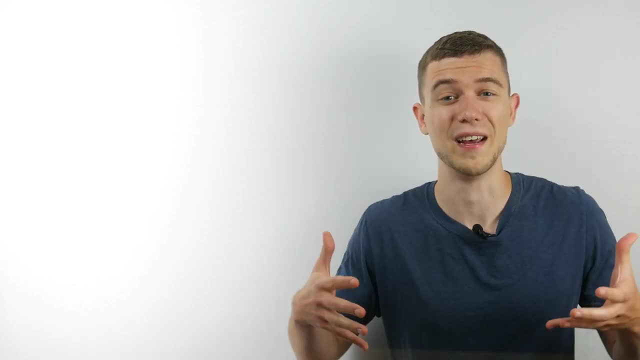 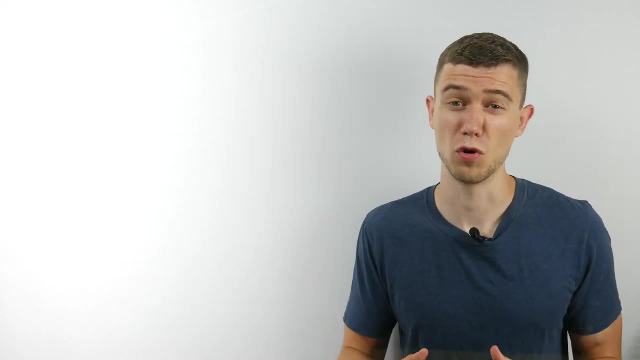 do themselves. you actually get to see students improve and get better grades and it's a really good feeling to be able to help people with a hard subject. it's very rewarding and i'm very glad that i am and will be able to be a tutor in the future, helping, hopefully, many, many people. i hope you like. 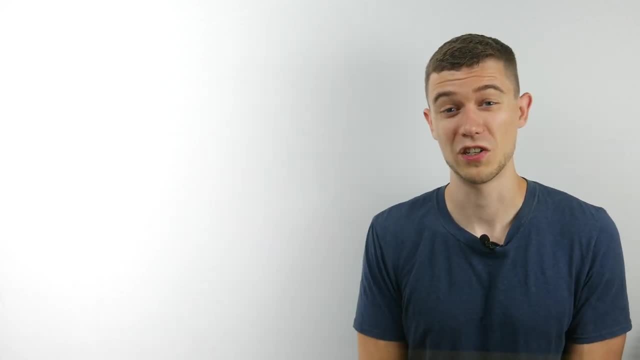 this video. i picked out this video for you to watch. if you're interested, i think you'll like it. it's a pretty good one. thanks for watching till the end and have a great day. 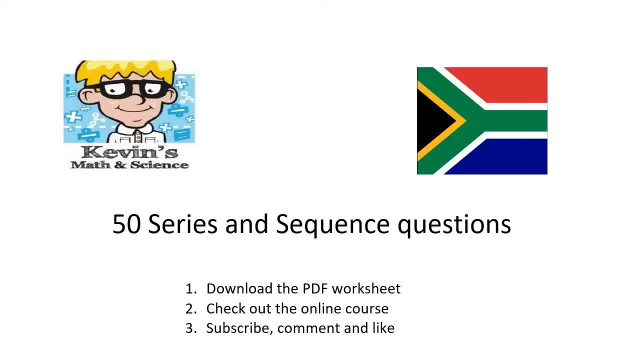 I'm super excited for this video. We are going to be doing 50 series and sequence questions. We are going to cover everything that you need to know in a series and sequence chapter, such as arithmetic sequences, geometric sequences, the sum to infinity. We're going to do a bit of 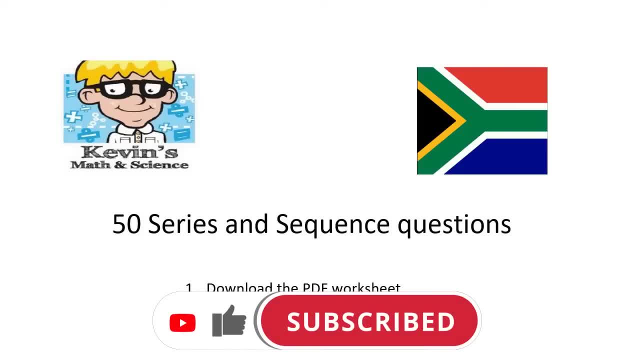 everything today. Before we get started, I would like you to know that in the description you can download a PDF, which is a worksheet that contains all 50 questions. This will be nice for you, as it allows you to see exactly what types of questions we are going to be doing. 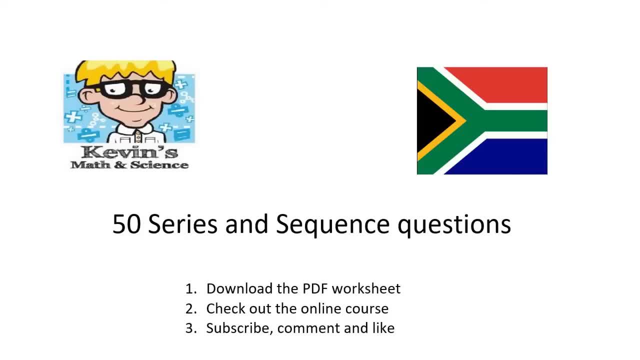 And so you can fast forward to the specific questions that you would like to practice. Of course, you can sit back and just watch all 50 with me, But for those of you who would like to go to specific questions, the PDF will allow you to see exactly what questions are coming up. 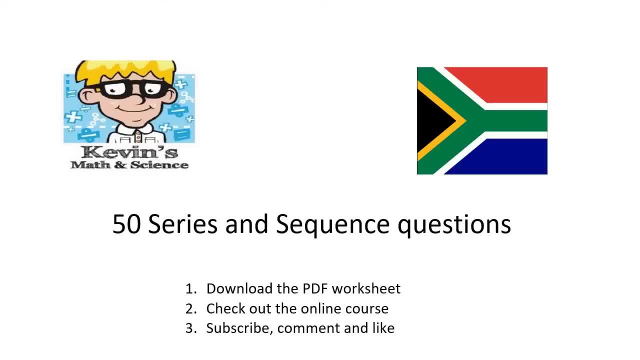 I've also added all the timestamps in the description so you can go to the specific question you are interested in. Did you guys know that I have a complete online course? The online course contains more than double the amount of content that I have on YouTube. 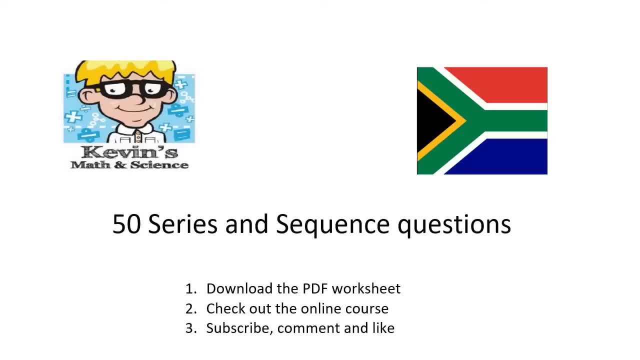 It's also organized way better. There's a question and answer section where you can ask students and you can ask me questions. There's an online community where you can chat to other students and get advice and help each other with maths and science. It really is nice. 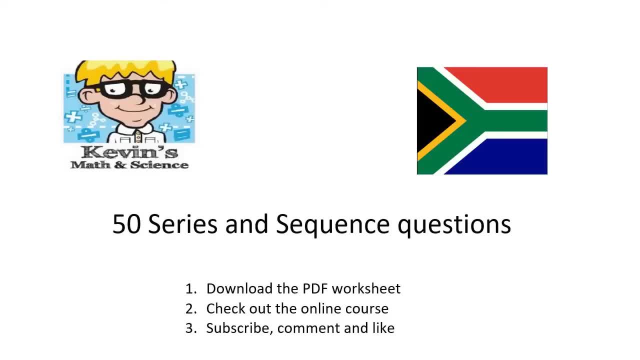 And then, lastly, if you are watching this on YouTube, please would you subscribe, leave a comment and like the video. You have no idea how the YouTube algorithm pays attention to the content that you are watching. If you are watching this on YouTube,